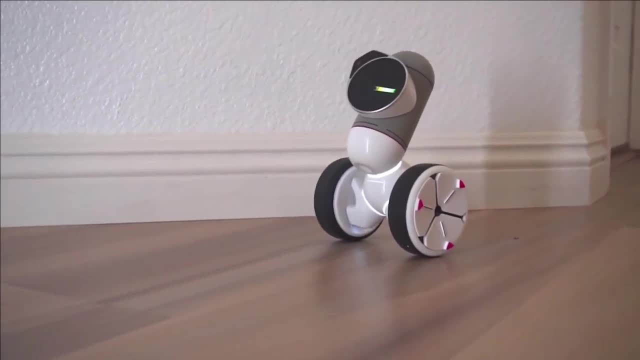 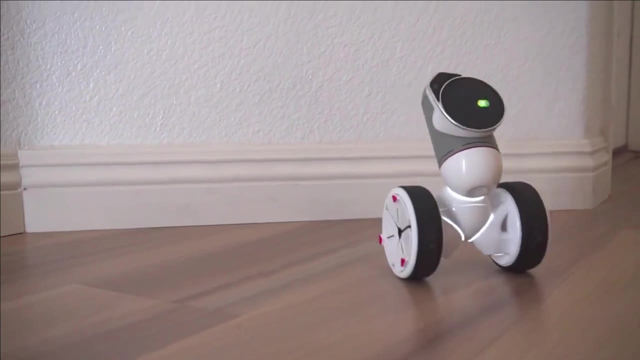 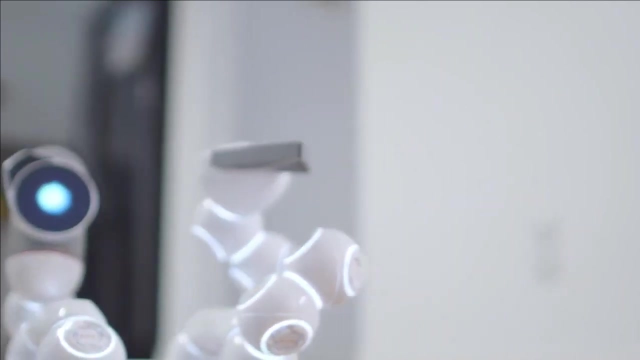 computers the ability to see, by building algorithms that process digital images or videos. It is mostly concerned with image classification, object detection and tracking and pose estimation. However, CV and its implementation in the robotics industry is multifaceted, which we will explore further in the coming sections. 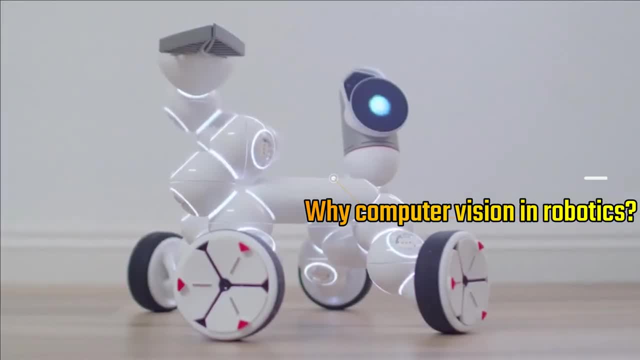 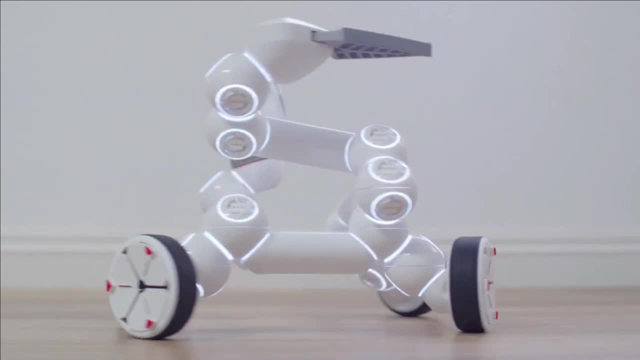 Why computer vision in robotics? If you still have a question as to why robotic vision is not enough, keep in mind the following: robotic vision can contain elements of CV And we know that visual data processing is a must for robots to perform instructions. 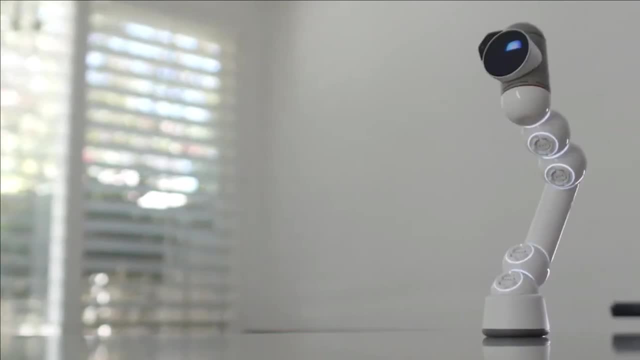 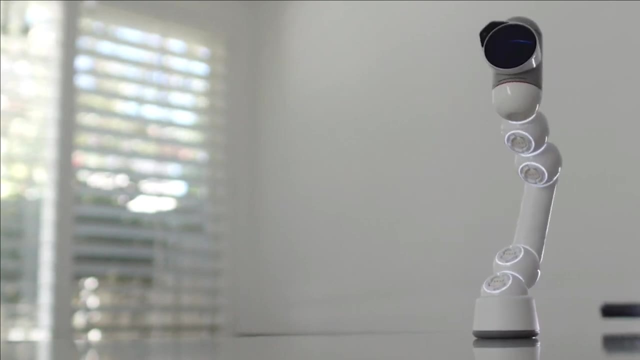 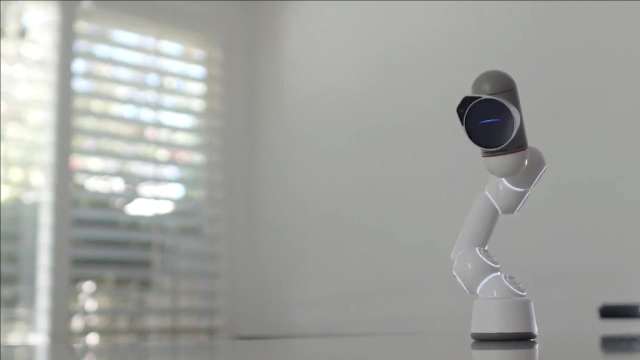 CV in robotics covers a broader spectrum of disciplines and reappears across categories From medical science and autonomous navigation up until nanotechnologies turn to robots to capitalize on daily operations. This points to the abundance of layers existing within the conditional CV applications in robotics heading Common applications. Visual feedback is essential. 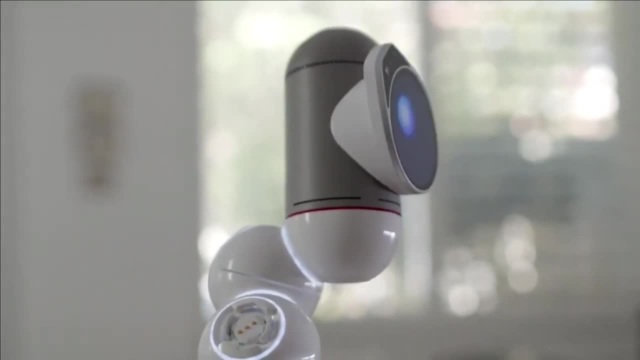 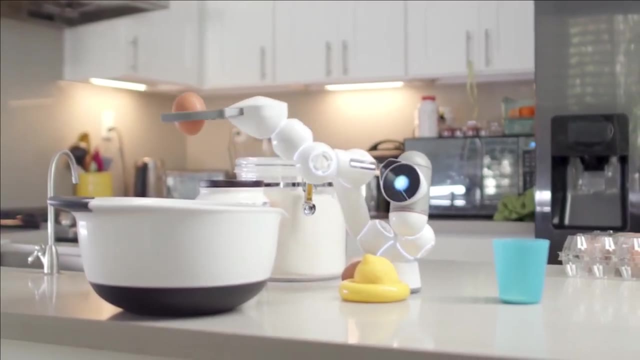 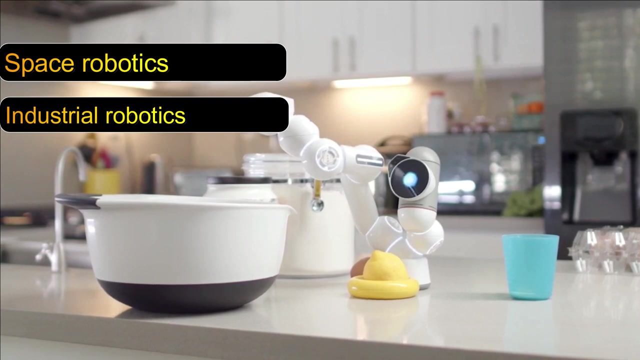 for image and vision-guided robots. Their power of sight is one of the elements that make them widely used across different disciplines. By and large, the applications of CV in robotics include, but are far not limited to the following: Space Robotics, Industrial Robotics, Military Robotics. 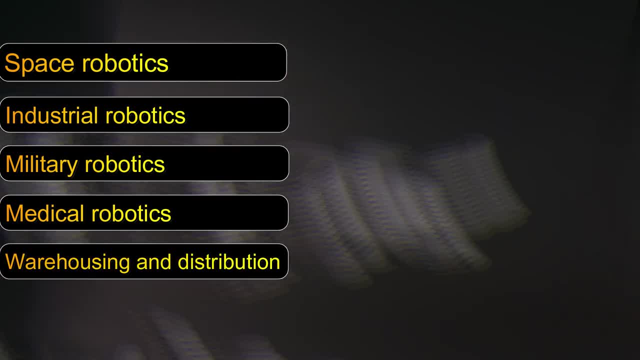 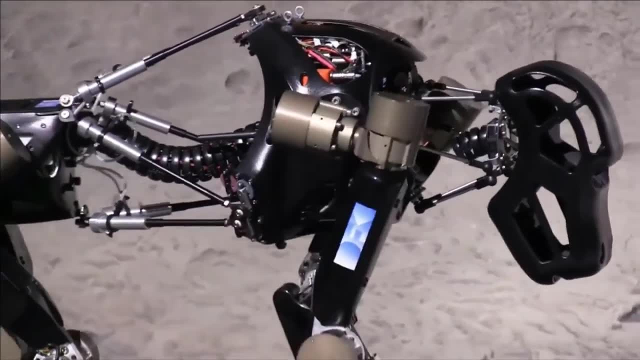 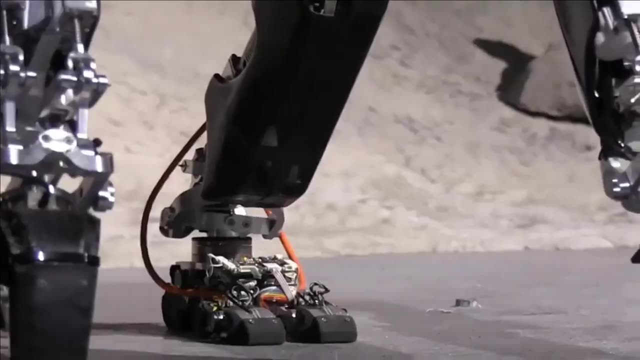 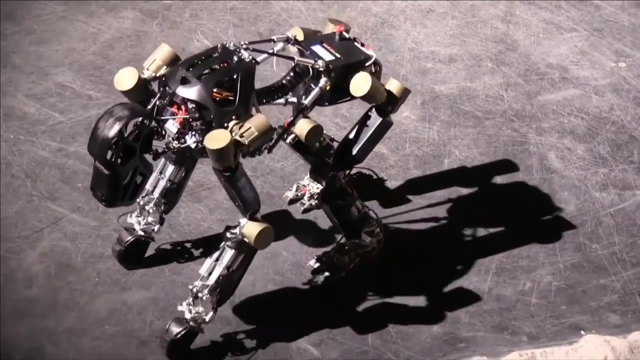 Medical Robotics, Warehousing and Distribution- Space Robotics. Space Robotics is quite a general category. It mainly covers flying robots that can be multipurpose and incorporate elements of on-orbit servicing, space construction, space debris cleanup, planetary exploration and mining. The main challenge for these robots is the continuously changing environment. 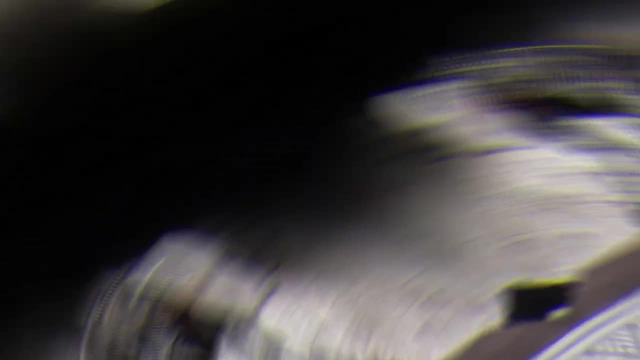 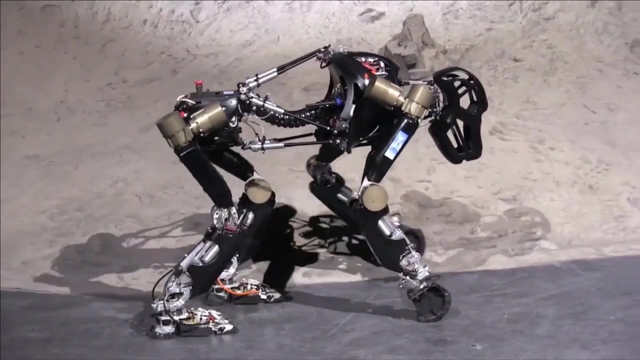 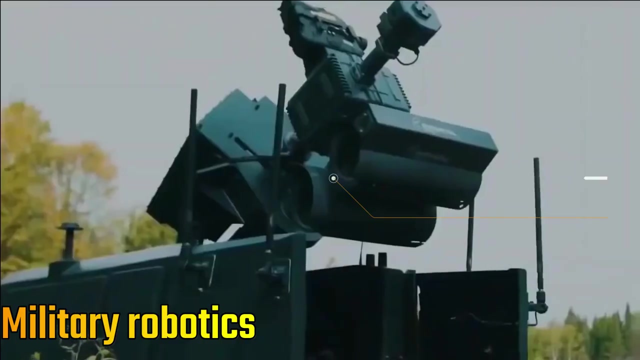 which hinders faster inspection, sample collection on a larger scale, colonization of celestial bodies and other activities. Although space initiatives are often quite ambitious, the use of CV promises streamlined solutions, even for space exploration purposes: Military Robotics. With CV integration, the door is open for robots to take on a broader range of tasks to assist. 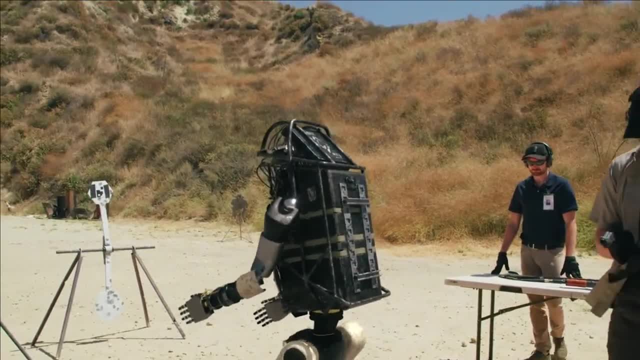 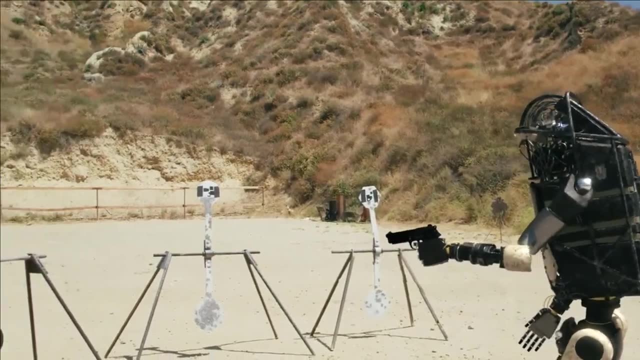 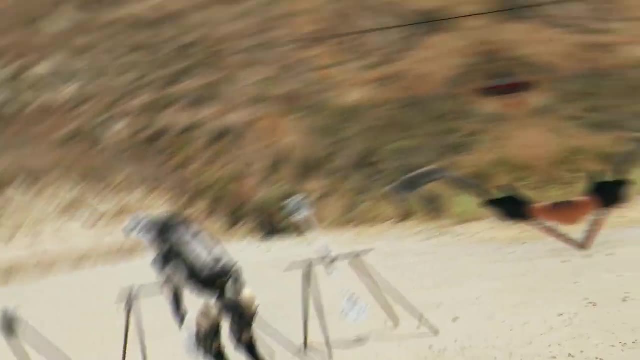 in military operations. The recent estimations confirm that global spendings on military robotics will be $16.5 billion in 2025, and for a good reason. the augmentation of CV into the military robots provides undeniable added value. Robotics went from luxury. 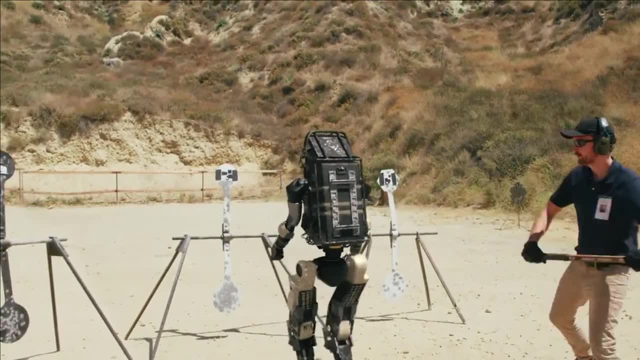 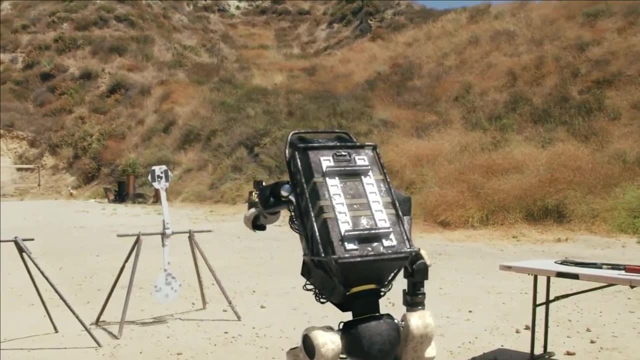 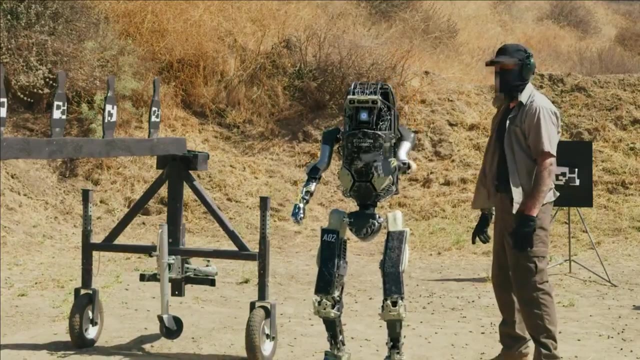 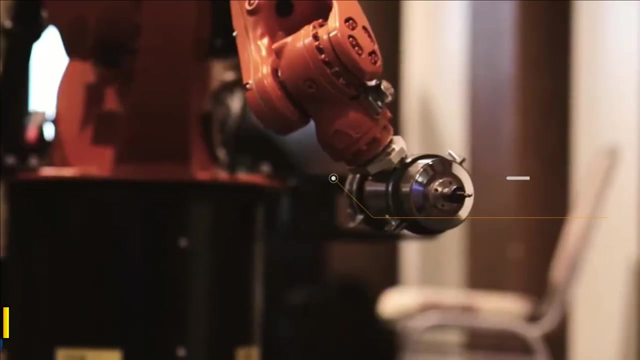 to a necessity, coming to the point where CV-embedded robot operations allow for the following: Military Robot, Path Planning, Rescue Robots, Tank-Based Military Robots, Mind Detection and Destruction. The latest generation of robotics promises more advanced functionalities and a wider spectrum of capabilities inspired by the human workforce: Industrial Robotics. 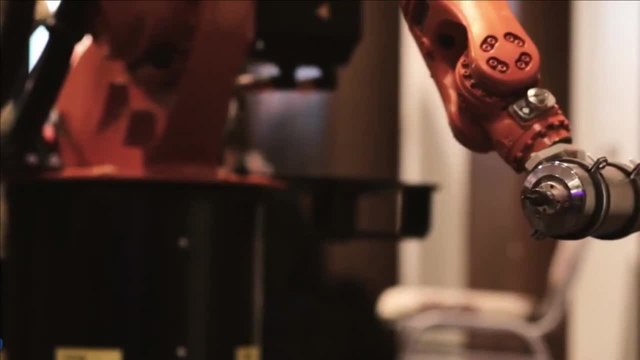 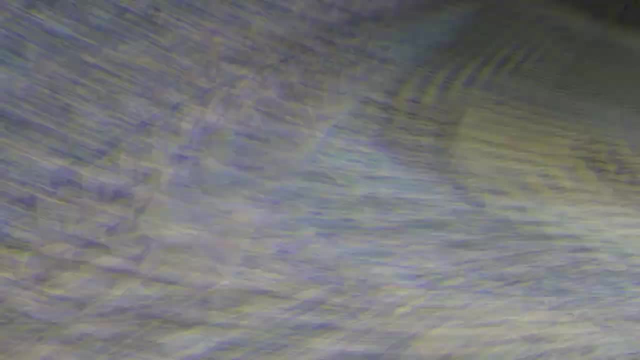 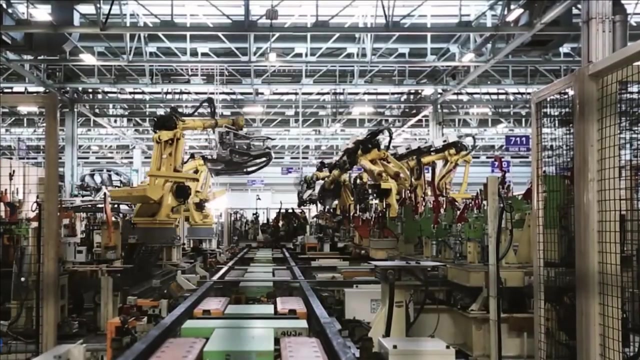 Within a few years, any task requiring human intervention can be partially or entirely automated. So it doesn't come as a surprise that the evolution of industrial robots pins hopes on CV. These days, the list of industrial tasks executed by robots is no longer limited to a robot arm. Odds are George Charles Devel, often referred to as 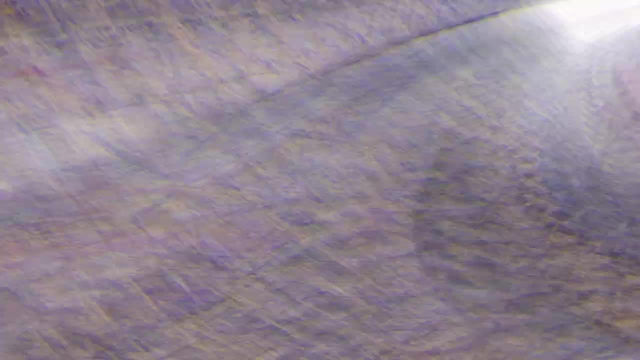 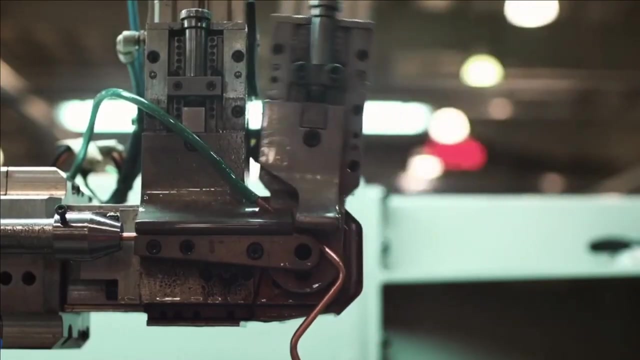 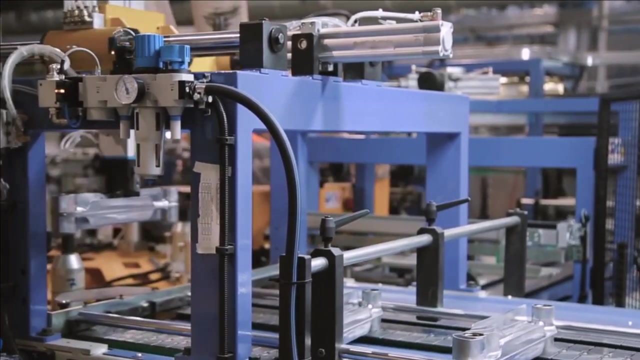 the father of robotics would be proud of this list: Processing, Cutting and shaping, Inspection and sorting, Palettization and primary packaging, Secondary and secondary Packaging, Warehouse order picking. Added to that, the increase of interest from industrial sectors in CV in robotics has many 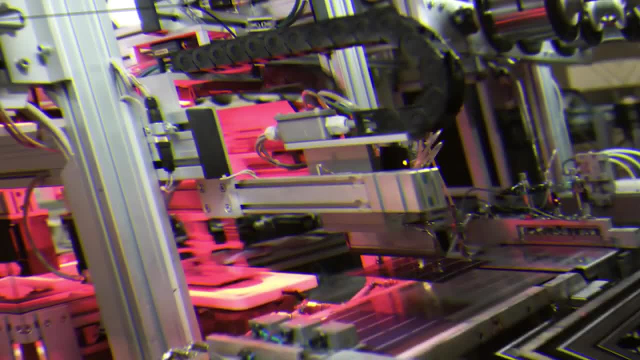 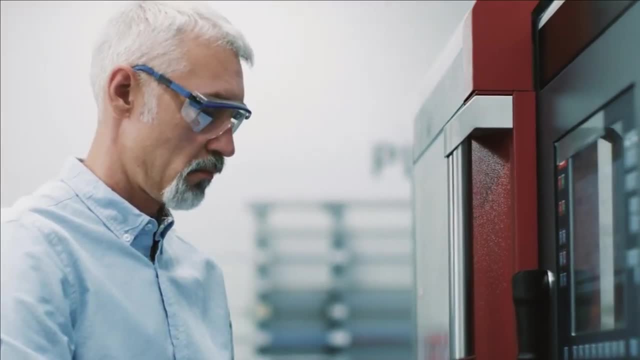 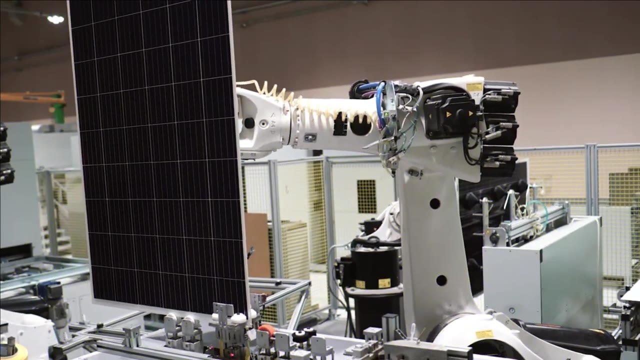 benefits –: first, robots reduce the cost for production long-term. Second, they offer better quality and increased productivity through RNA. Thirds, they enable higher flexibility in production and respond to the shortage of employees in the fastest way possible. The drivers above trigger trust and further investment in robotics and CV-inspired 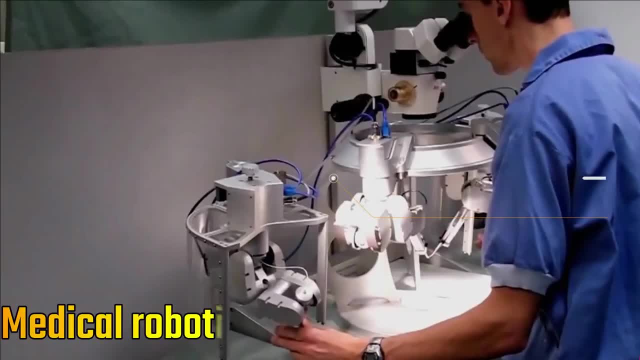 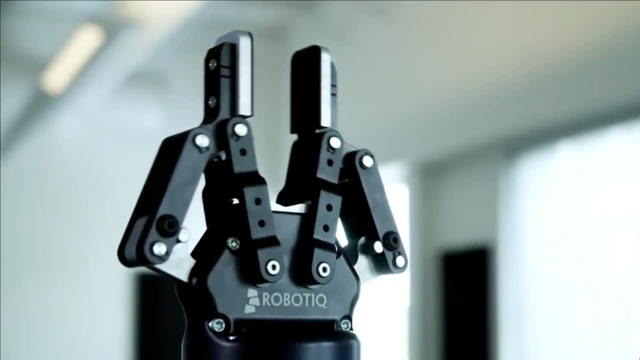 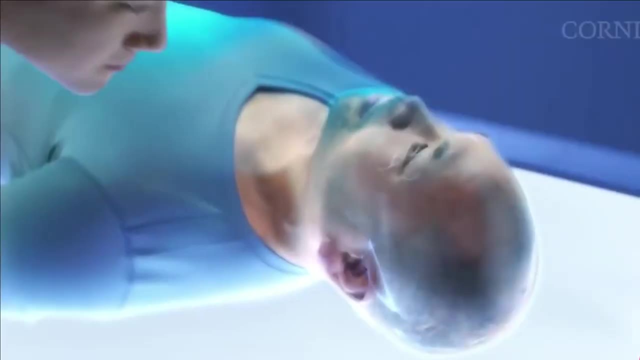 automation solutions in the industrial sector: Medical robotics, The analysis of 3D medical images by CV fosters diagnosis and therapy. but CV applications in medicine do not end there. Robots are especially helpful in surgery rooms, fulfilling operations in three categories: pre-op analytics, intra-op guidance, intra-op verification. To be more specific, 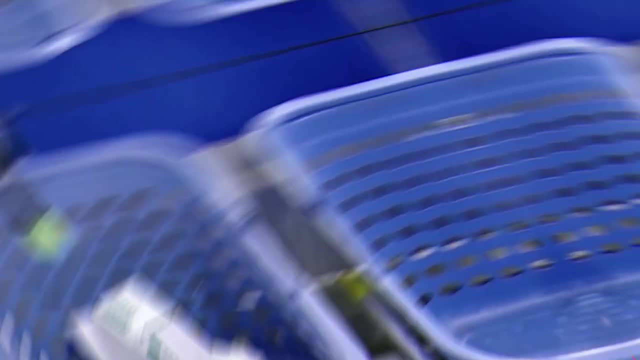 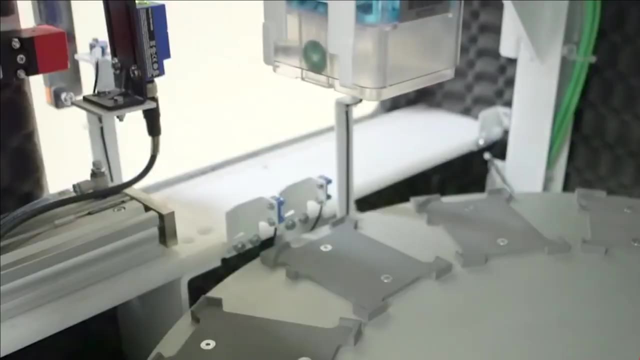 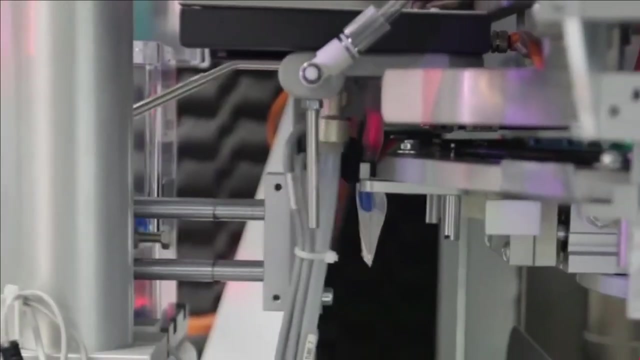 they can use vision algorithms to do the following: Sort surgery tools, Stitch tissues, Plan surgeries, Assist diagnosis. Short and on point, they make sure that the surgery design and respective steps match the actual implementation for the brain, orthopedic, cardiac and other. 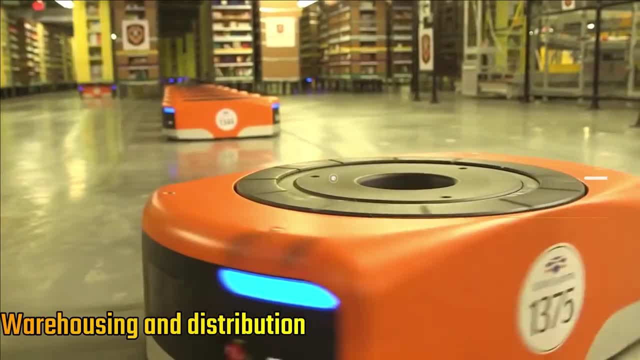 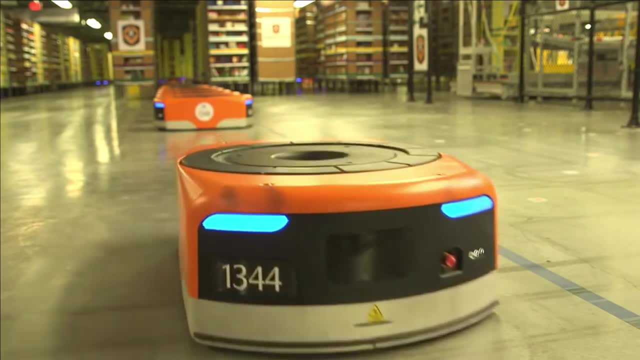 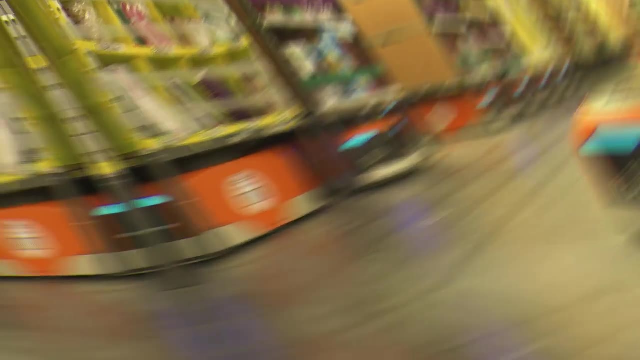 surgeries, Warehousing and distribution. As more people shop online, the not-too-distant past of warehouses and distribution centers turned to robotics solutions to automate picking, scanning the barcode, tossing the products and other stages of distribution. Standing all day to sort and pick goods is neither convenient nor efficient in this day and age. 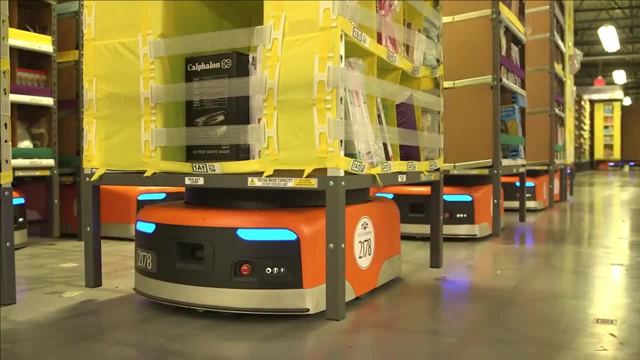 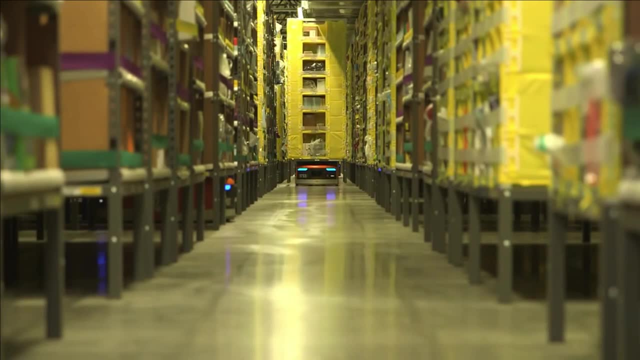 To bring an example from one of the leading players, Amazon purchased Kiva Systems. yet in 2012,, to be able to move shelves of products without human intervention, Soon, FedEx and Okato also turned to their own AMRs. years later, and these were only the first waves. 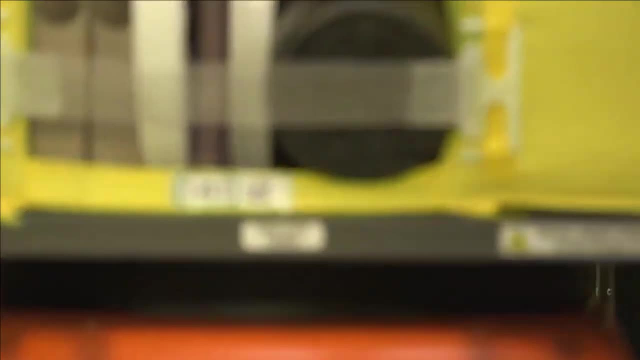 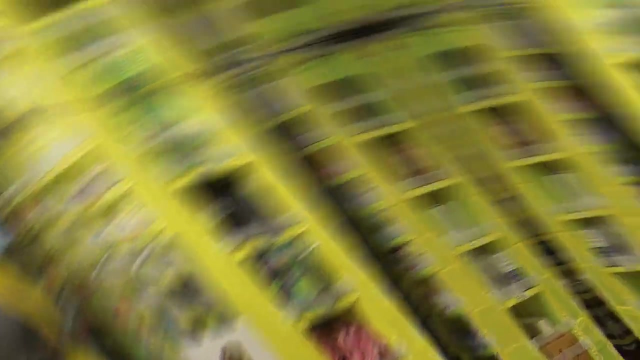 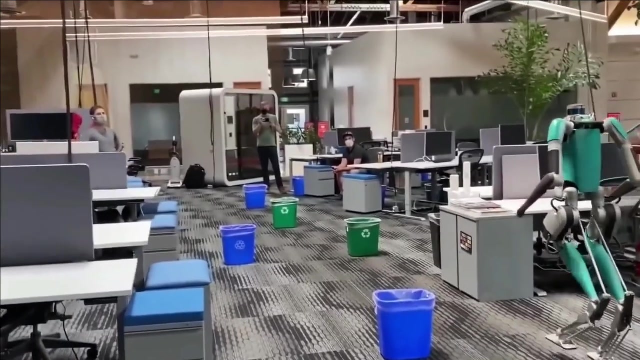 of automation. Drawing parallels with today. moving objects from one shelf to another is one of the most primitive robotics challenges, and there's still a way to go to completely automate the warehouse and distribution industry. Computer vision challenges in robotics. The next generation of robots is expected to overrun their traditional counterparts in terms. 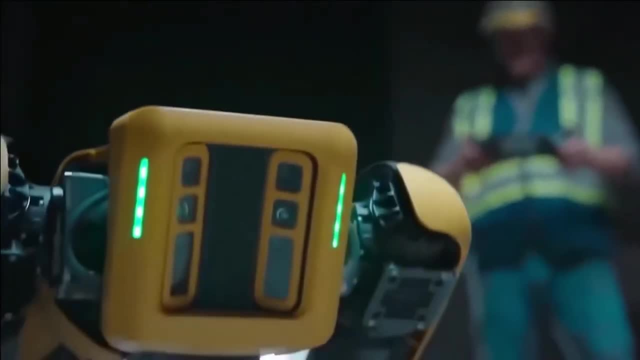 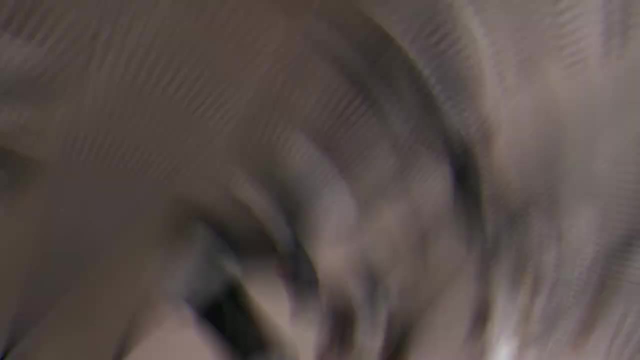 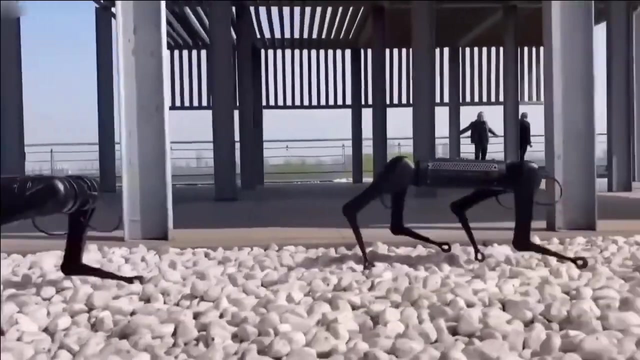 of the provided skill set. CV and robotics combination is already a huge step forward and is bound to transform the technology. However, the abrupt advance in automation and the increasing demand in collaboration with humans pose several challenges for CV in robotics Identifying moving objects. it's integral to consider three situations when it comes to robot movement. 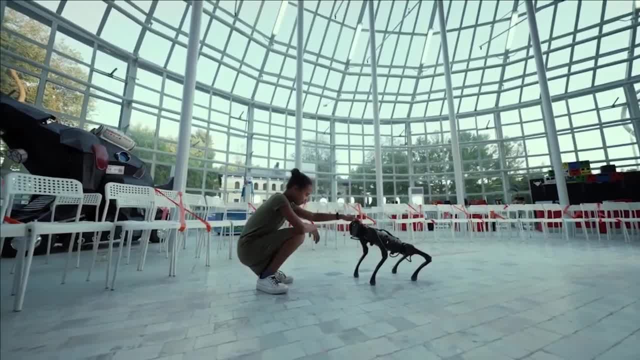 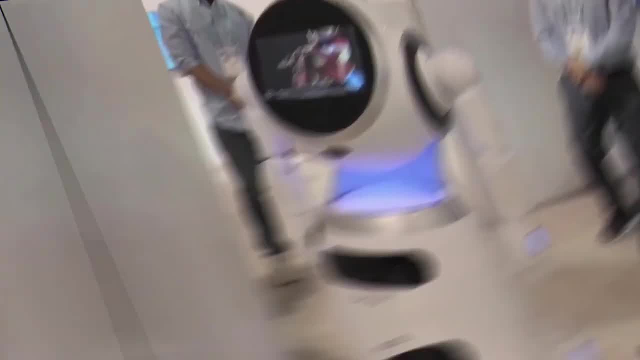 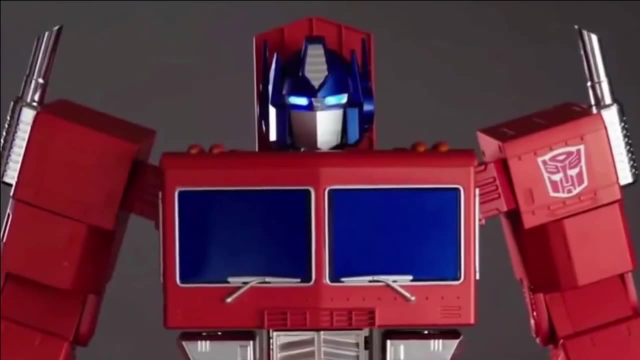 The robot is moving and the object is static. The object is static while the robot is in motion. Both the robot and the object are in motion. Making sure the robot operates in content with all three situations is time-consuming and costly, yet makes up for the effort, providing higher. 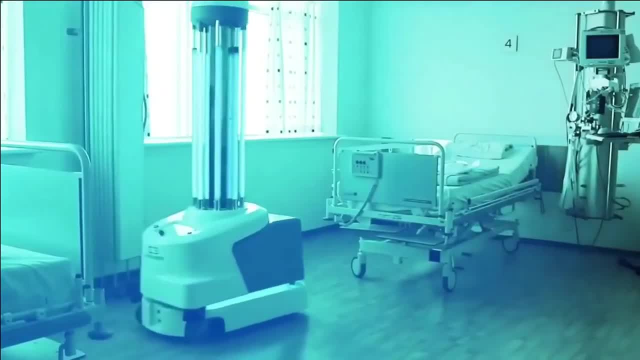 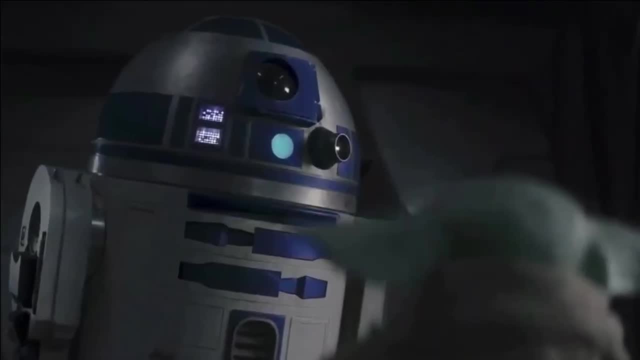 levels of performance: accuracy: Identifying covered or partially visible objects. occlusion when the target is not visible on the screen. Identifying covered or partially visible objects. frame and cannot be detected is quite common in robotics and CV To combat occlusion. 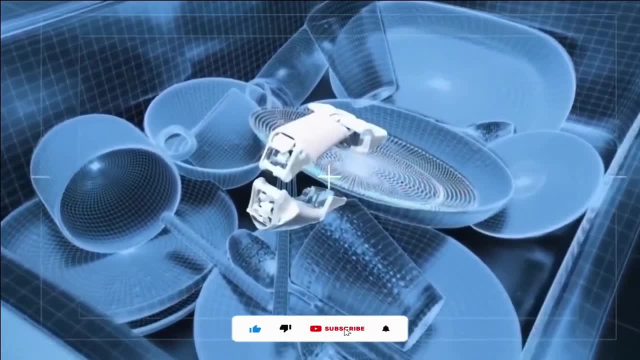 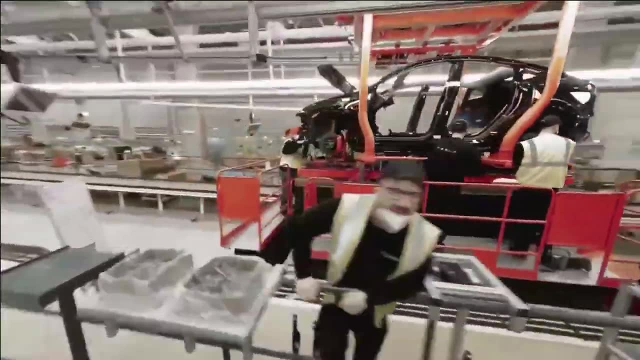 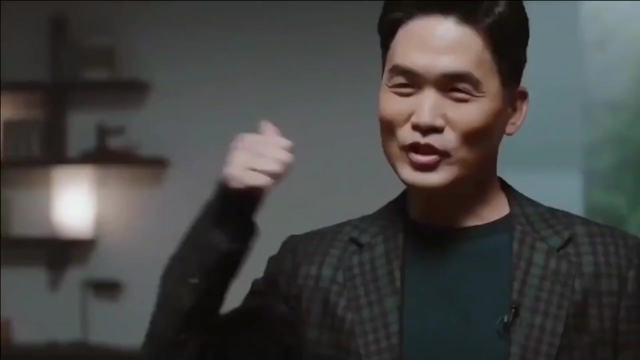 it is significant to build an algorithm that connects the visible part of the desired object with the stored image, Recognizing deformation and modified shapes. robots will have problems detecting deformed objects without an advanced visual mechanism. Being able to detect crashed vehicles, for instance, can be pivotal, especially for the automotive industry and defense. 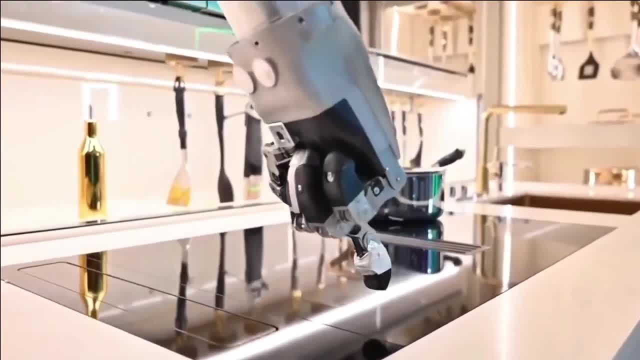 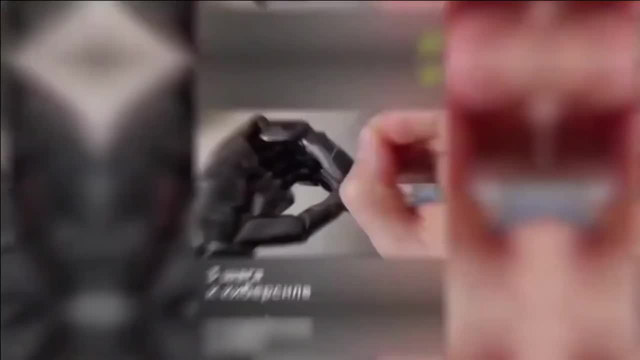 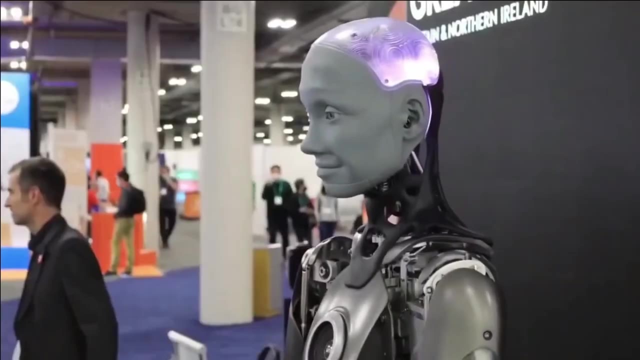 Recognizing the position or orientation of objects. robots require a comprehensive sense of orientation to perform one of the primary tasks in manufacturing or industrial robotics: pick and place. Identifying 3D orientations can be especially challenging due to the lighting conditions, the difference in colors, texture.